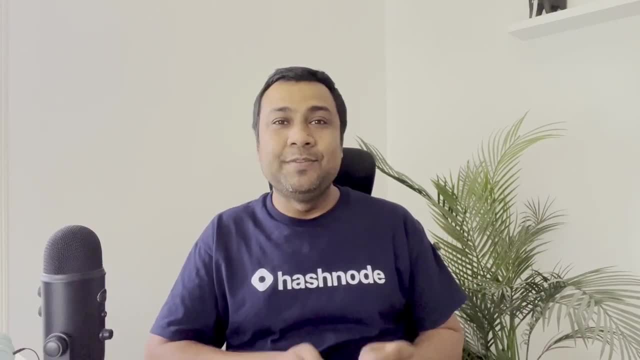 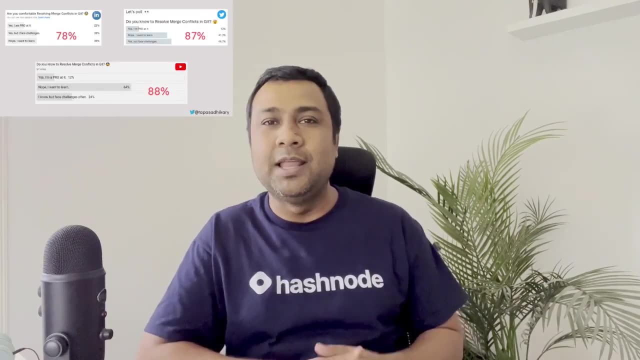 Hello people, how are you doing? Today we are going to discuss about a very special topic: resolving merge conflicts in git. Very recently, I have taken a survey on various social media platforms like twitter, linkedin and youtube. So what I found? I found that most of the people 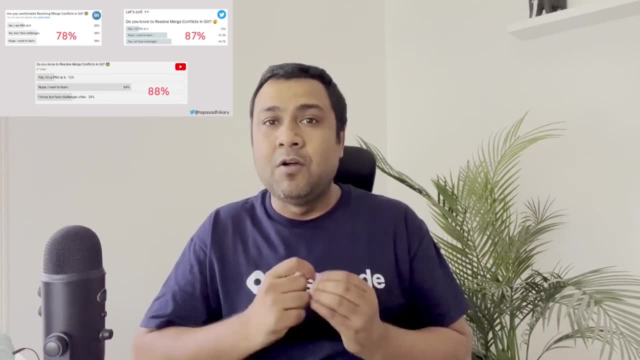 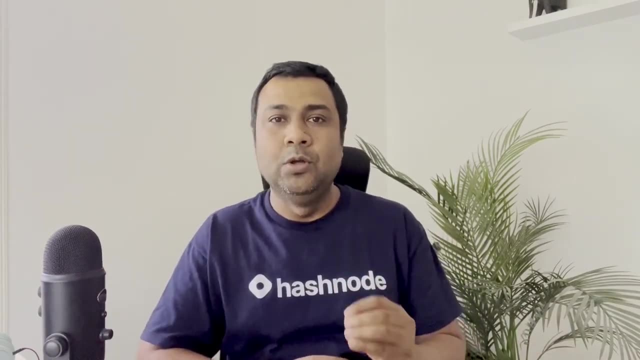 acknowledge that they face challenges in terms of resolving merge conflicts in git in a correct way. So I thought, why not to make a very short video about it so that I can actually take you through with lot of examples of how to resolve merge conflicts in git. Resolving merge conflict in. 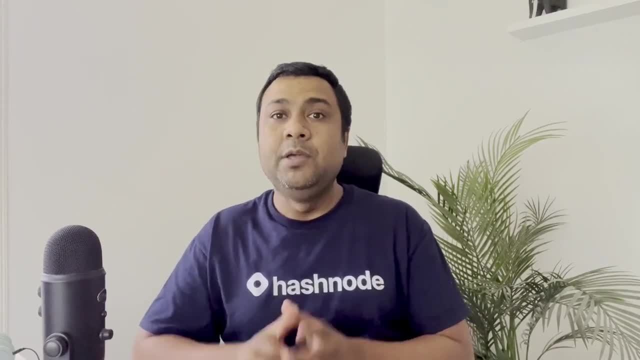 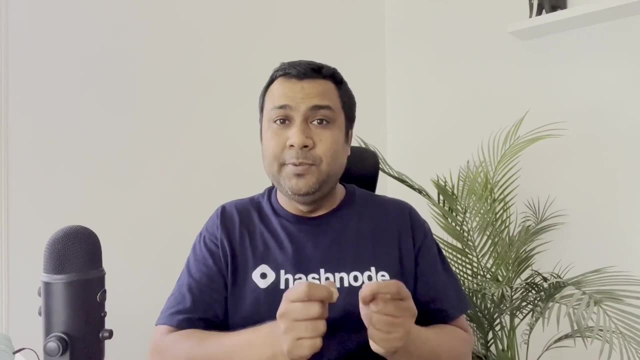 git not only about the technical perspective that you have to think from. you also have to think from like what is required for your project and, based on that, you have to take the call All right. so in this short video, you are going to learn all that, and I want you to practice as. 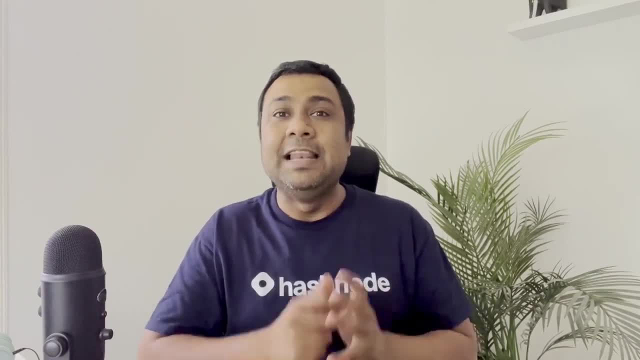 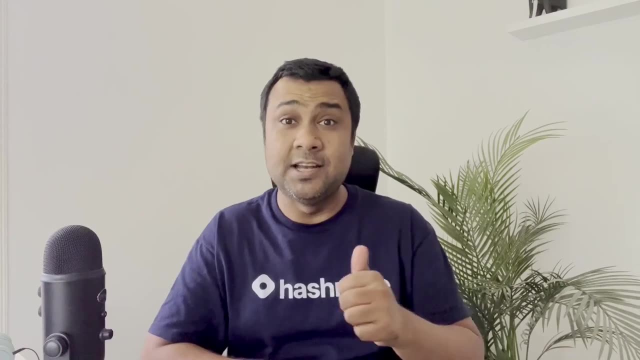 you are going through this video, All right. so, without any further delay, let's get started, but before that, don't forget to subscribe to this channel, because we keep sharing, love and support A lot of great content in this channel. All right, so let's get started. 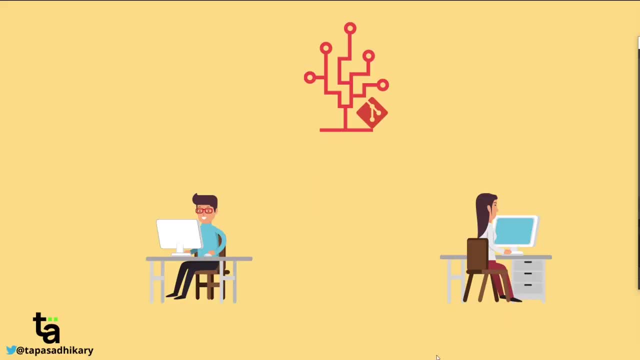 Do you like stories? I have one story to tell. So let's consider two individuals You know, one is Alex and another is Tina. They are working in an organization, working on the same code base that is hosted somewhere at the remote- maybe github. In their daily life they are as they're. 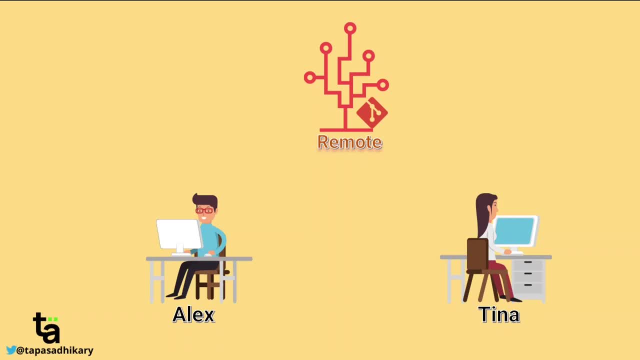 working on the same project, there are higher chances that they will be touching the same files individually. So on a fine day, what Alex is doing? Alex pulling some changes from the github or the remote to his local and then making some changes into the abctxt file and then pushing it. 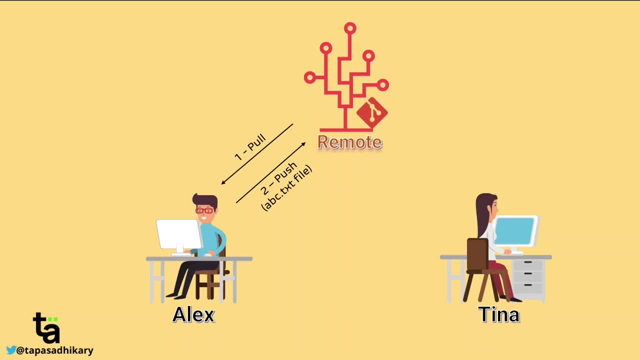 back In the same time on this. you know, Tina, without being aware of that, what Alex has done in the abctxt file. she also made changes in the same file and trying to push it, but as her changes, her changes, are kind of a bit behind than what Alex has done, and git being a version control. 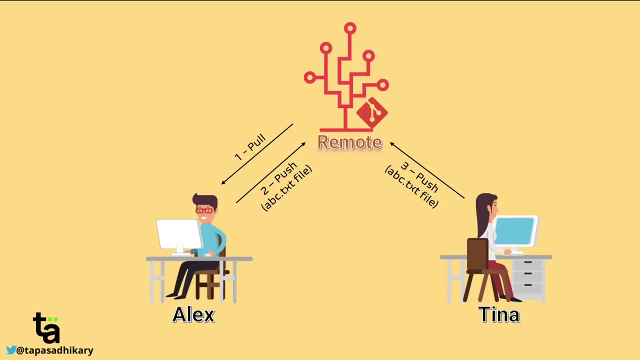 system always keep track of each of these files. in changes in terms of versions, It is going to reject that particular push. So what Tina understand from this one? hey, probably somebody has made changes into this file- abctxt file- so I have to first pull the changes from. 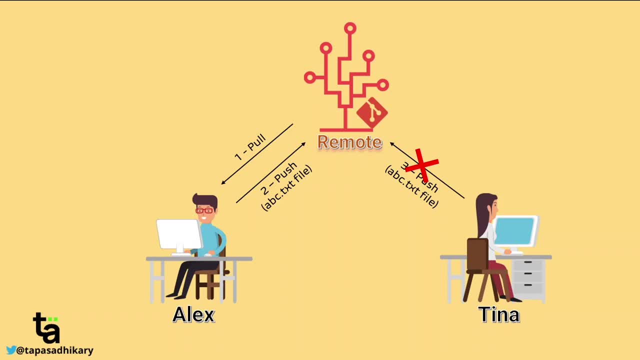 remote and then see what changes has been done and then I'll be finally pushing it. So with that hope she pulled the changes. but once she pulled the changes, what she gets? she gets merge conflicts and as Tina gets that now Tina has to fix the merge conflict. We will get back to this story. 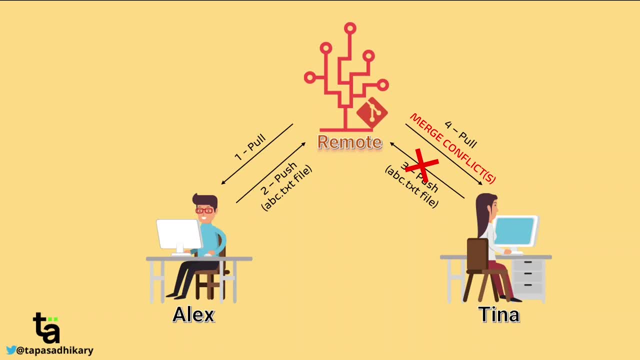 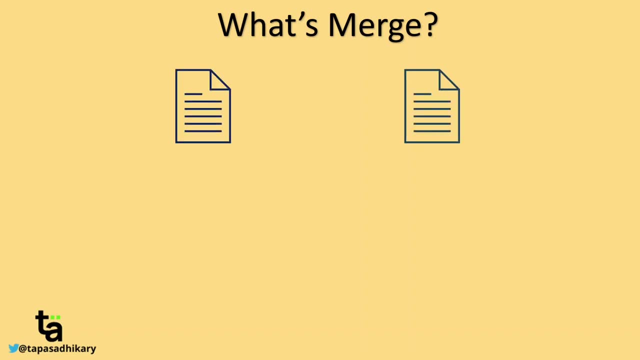 but let us understand what exactly merging means and why exactly merge conflict arises. So what is merge? Git is a version control system. so it means that for a single file there will be multiple versions. One version could be created by my friend, another version could be by me, another. 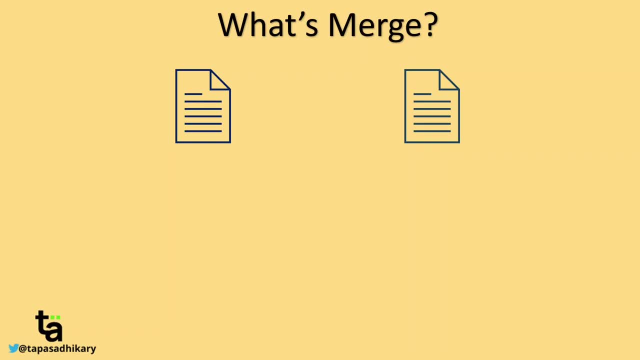 version could be somebody else and they would have changed the same file, done the same, some kind of modification into it. Ultimately, all these versions has to be merged and create a new version, which is the latest and greatest that somebody has to start working on. By the way, if you don't understand some of these terminologies or you're just getting started, a 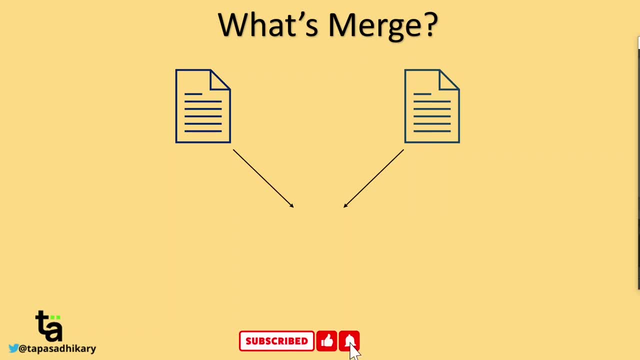 beginner with git. I have already created a video for git basics for beginner, so you can just go ahead and have a look into it. I have posted the link of that video into the description of this particular video, so go ahead and catch that particular video. Alright, so coming back to 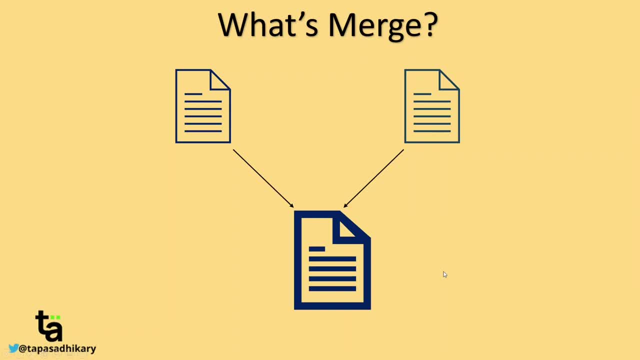 this one, a merged file. a merged version of the file will be created. So when a merged version of the file gets created, there are two things happen. One is changes and the other is possibilities. So what kind of changes in a merged file can happen? The changes can be. 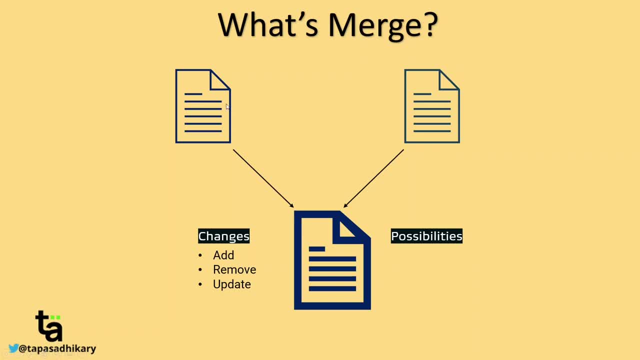 add, update or remove. It means that from this particular version, from this particular version, there could be something got added or something got removed or something got updated, right, and then these two things got merged and then created a new file. Now, when these changes happen there, 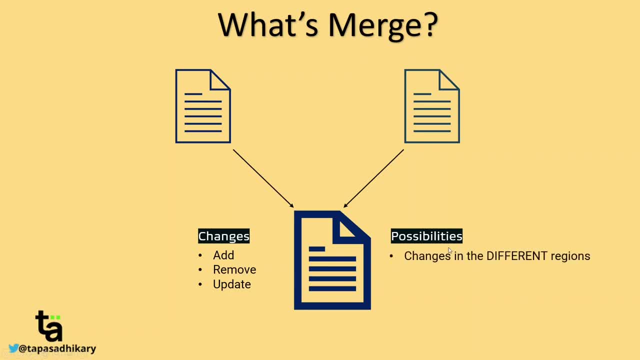 could be two possibilities. These changes that I have just now spoke about- add, remove and update- would have happened into different regions. It means from this particular file, the changes some would have happened at the top, this particular, another version of this file, the changes would have happened at the bottom. So if I just merge these two, one changes at the top, another change. 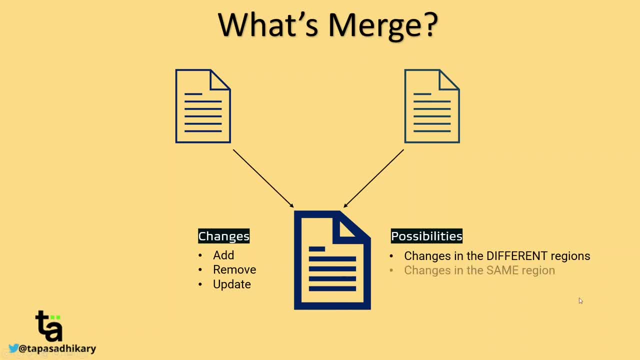 at the bottom. Okay, so it's a different region of the file. Another thing can happen is in the same region of the file. So, for example, in some version this particular line has got updated, or the other version, the same line, got updated. Now again, if we are merging, then this update has. 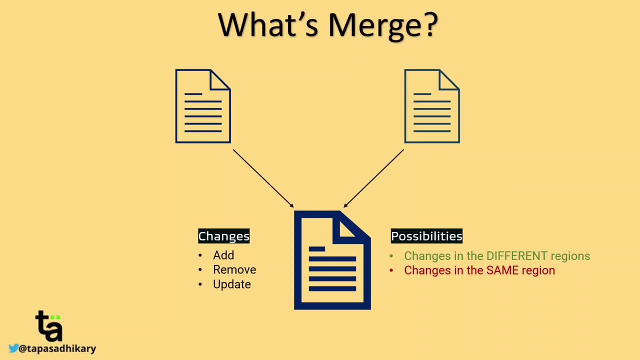 to take care of. Now what git can do, Git can actually tackle the changes in the different regions by itself while merging, Where git don't take the decision if the changes in that different, you know in the same region. So in that particular case git doesn't. 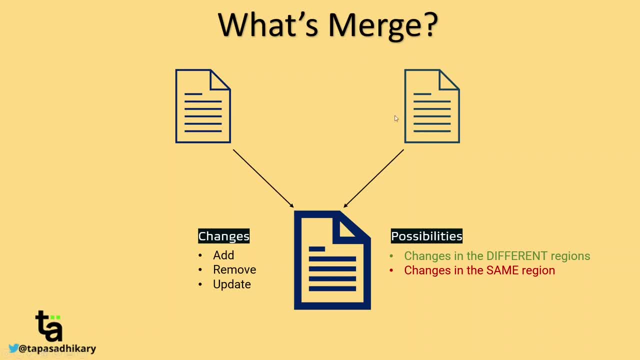 know whether I have to take keep this change or keep this change or have to keep both the changes. and that is the time the manual intervention required. That is the time you have to resolve merge conflict as a developer. So I hope you understand this thing. 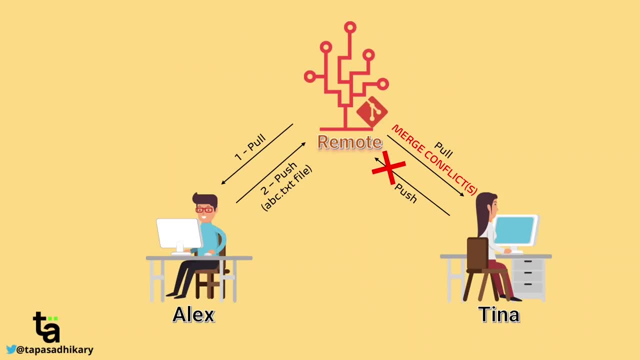 Now let us get back to our story and see what Tina is going to do. So first, Tira, What Tina is going to think. Tina is going to think: hey, what should I do? Should I remove Alex changes and keep mine, or should I keep Alex changes and remove mine, or should I keep both the changes? 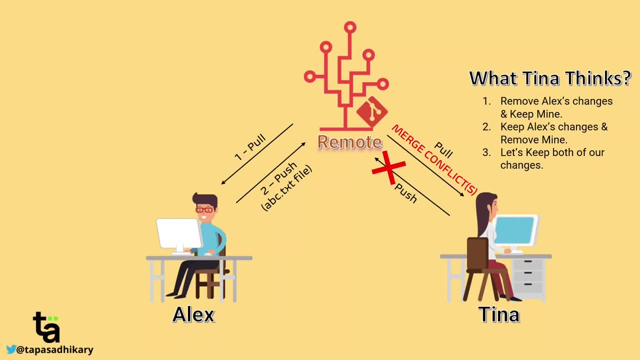 or another possibility would be: should I remove? you know both the changes, So what exactly Tina should do, it all depends on what is the use case of the application they are working on. If something like that, Tina feels that, hey, Alex, changes is no more valid after my changes, so I'm going to remove. 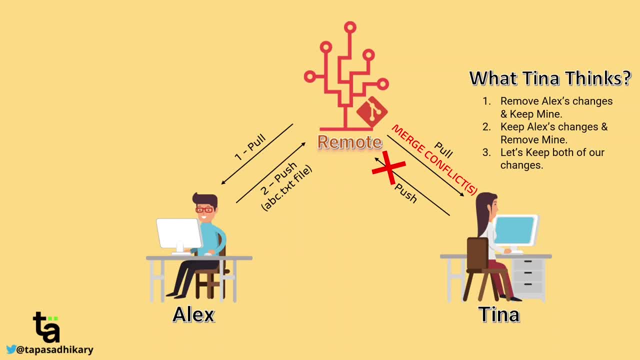 Alex changes and just keep mine, or both the changes are valid. I'm going to keep both or I'm going to remove both. that call that Tina has to take. That's the manual intervention. That is the manual intervention thought process of resolving merge conflict. Once Tina decide. 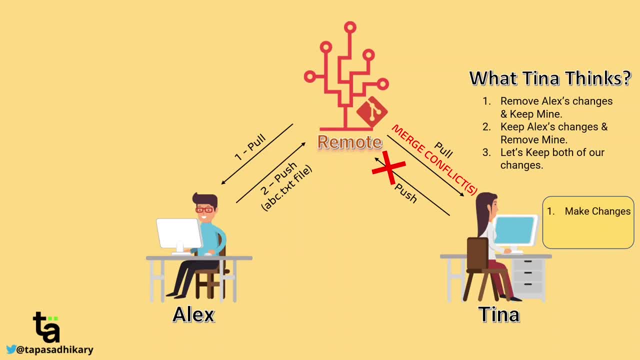 that Tina going to perform few steps. One is Tina will make changes based on the decision she has been taken. Then she will stage the changes. It means she will do the git add of the file Again. if you are new to this, please go through the beginners video first so that you understand. 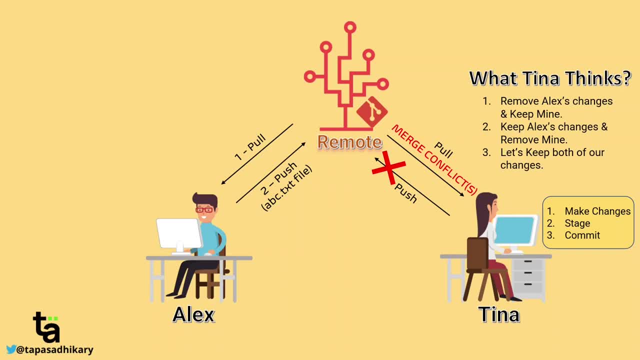 these terminologies. Then, finally, Tina is going to do a git commit. Now the thought process, the git taking and doing all this thing together is called resolving merge conflict. After this, only merge conflict is going to get resolved. Then, finally, what Tina is going to do, attempt another. 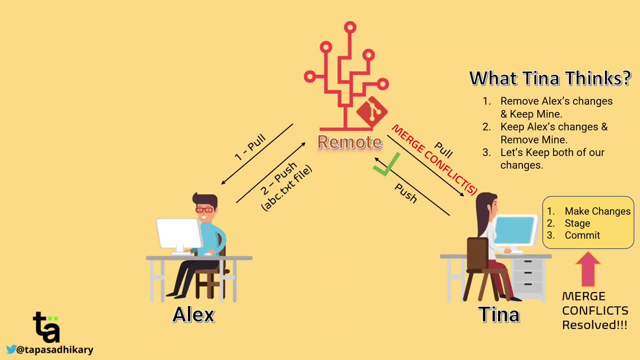 push, and this time the push becomes successful. So this is the story, guys. How was the story of Alex and Tina Now, if you understood that story and if you face this story in your daily life, what we're going to do now, we will see practically how to tackle certain situations when we get merge. 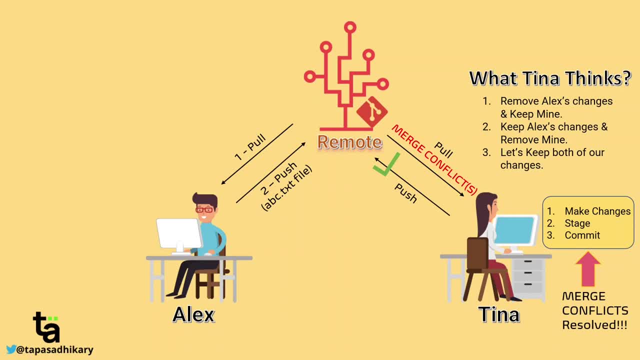 conflict. You up for that? Okay, so let's get started with that- and where we will be seeing some of the situations. We'll be learning from it. I would like to request you to come back to this video, the portion of it where we'll be showing example, and try out by yourself. then you will learn it much, much faster. 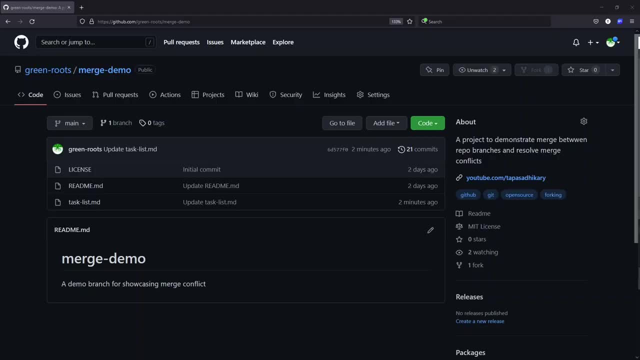 Okay, so let's get into the examples right away. Now we will learn from the example. For that I have a repository called merge-demo with bunch of files over here. One of the file that we are interested in is called task-listmd. Let's go to this file and see the content It has only 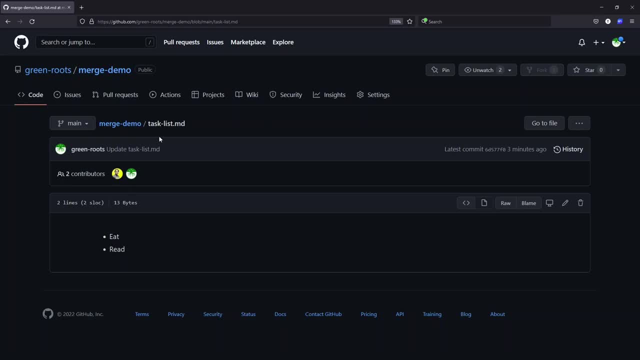 two bulleted points. one is eat and read, And this particular repository called merge-demo is under the account called green roots. Okay, now what we'll be doing is like we'll be making some changes to this file and from another account, we'll try to make the. 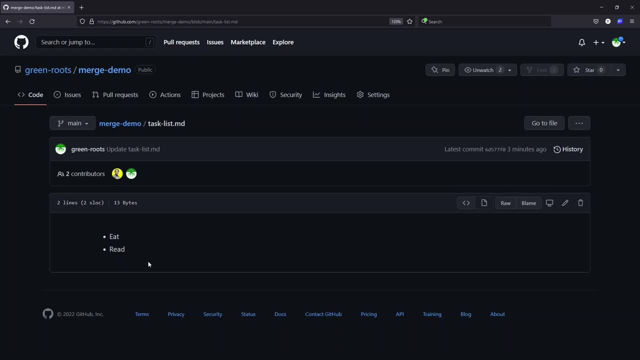 changes to the same file and try to create a situation of merge conflict and then try to resolve that. Okay, so first thing. first is like I'll be making some changes to this file Now I'm making these changes directly from the GitHub because to just for the demo purpose. So eat read. 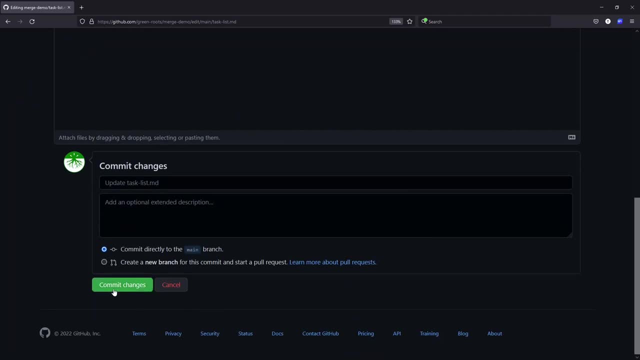 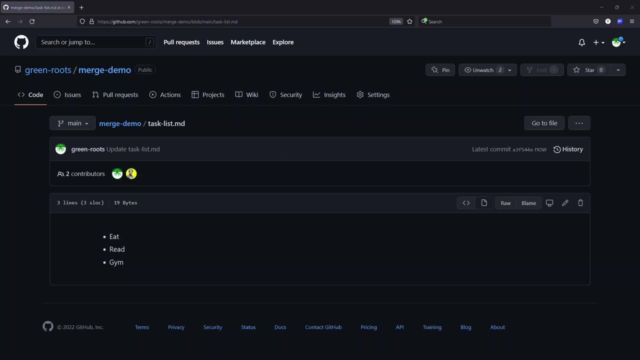 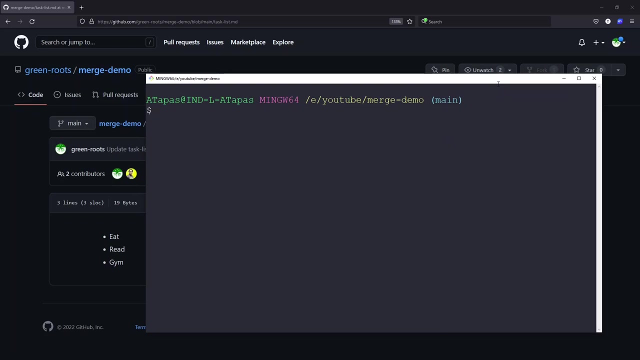 gym, and then I'm going to update this file directly into the main. This is only for the demo, don't do it for your actual project. So I see, eat, read and gym is there Now in the command prompt. you know my hard drive. I have actually cloned this particular project, as another user called athapus, which is my 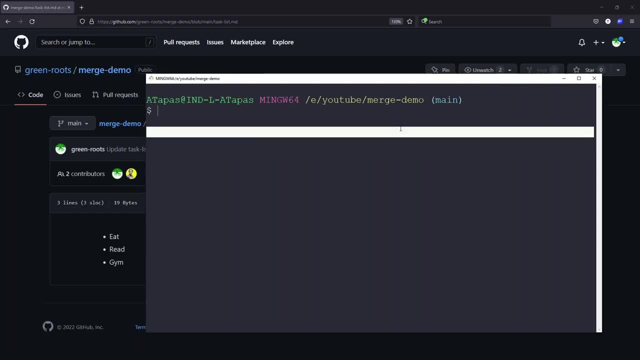 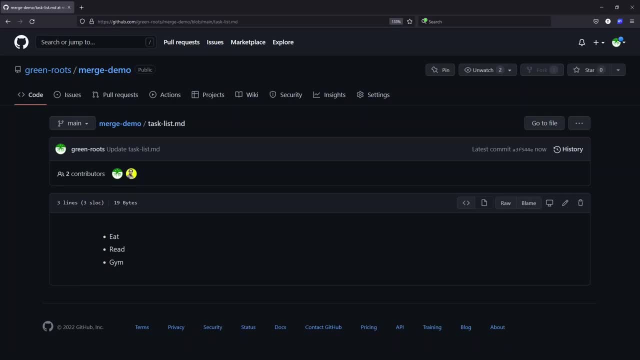 account. Okay, so here, what I'll be doing now is like I am going to make some changes without being aware that green roots have already made changes into this file. I'm making changes to the same file, So I have my editor over here and I'm going to say: slip, Okay. 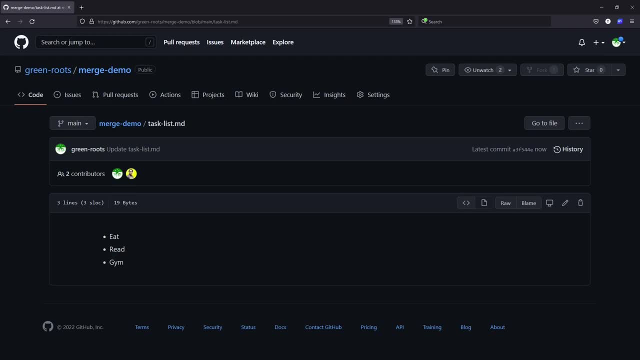 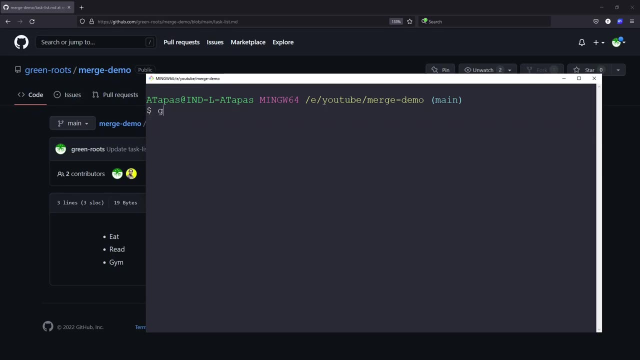 so I have made some changes called slip. As the changes have been made, the next thing that I am going to do using my git bash, I am going to straight away going to stage these changes. So first I will do git status. I do this git status always is kind of a habit to check, like you know. 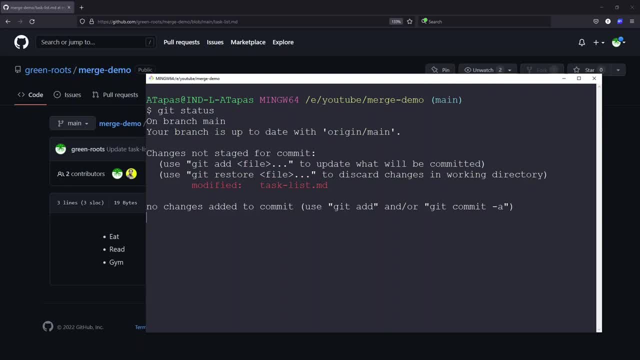 what are the files? got changed by me locally, So this is called task-listmd. has got changed right file. Let's stage it Using git add task-listmd command. So it's taking some time, Yeah, so git add task-listmd. 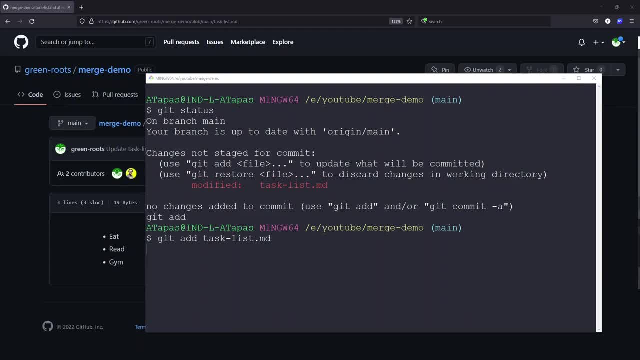 So this will go and you know: do the staging. The staging is done. The next thing we'll be doing a commit. So do a git commit, minus in added task a commit message and I press enter. It should get committed. The commit is done. Now the next thing would be like git push origin main. So I'm 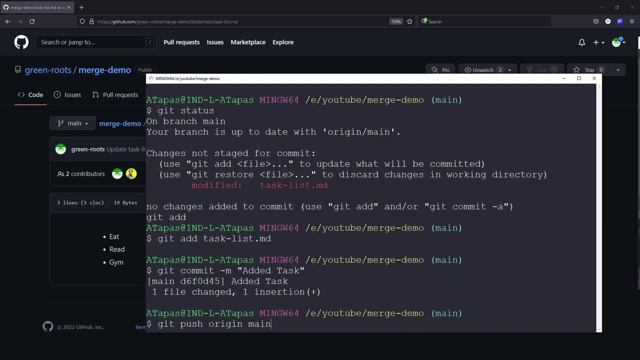 pushing to the remote my changes. Now, if you notice over here, this is: this: push is being done by athapus, another git user, on the same file, on the same location that green roots have modified. Now athapus doesn't know that green roots have modified. Now what we'll be expecting? an error. 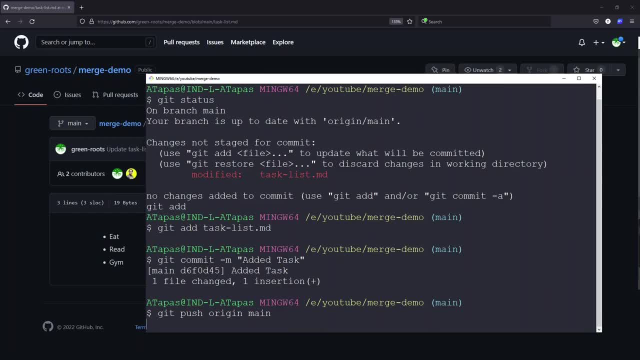 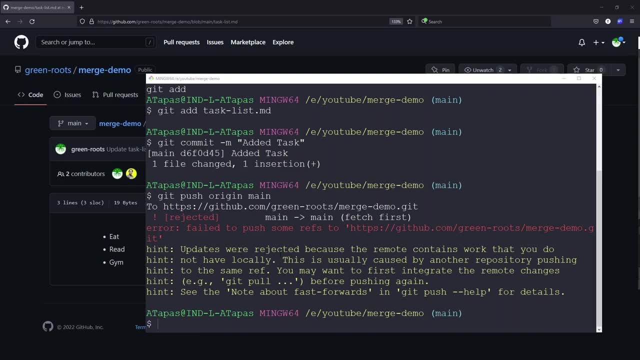 by git saying that your branch is behind. First you pull it before you make any changes and push Okay. so let's see that, As expected, I'm getting an error, fail to push, The reason being: it is rejected because remote contains work that you do not have locally, So you have to pull Now, athapus. 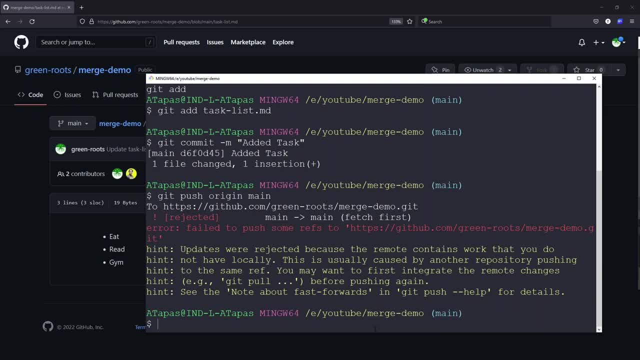 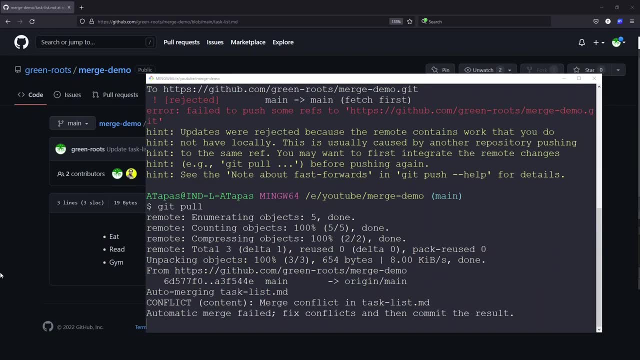 again, without knowing that some you know what kind of changes would have happened over here. We'll go and pull the changes and this is when our merge conflict may arise. Okay, what do we see? We see like git is trying to do auto merging, but this auto merging has failed. 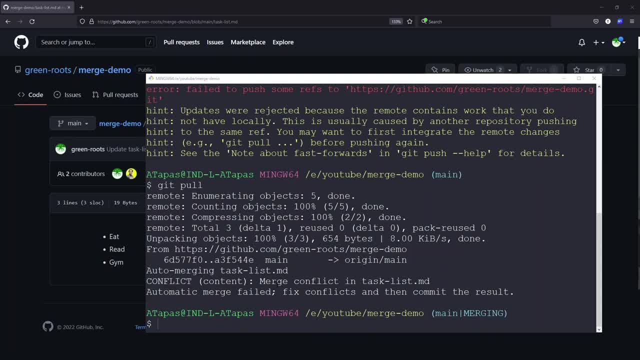 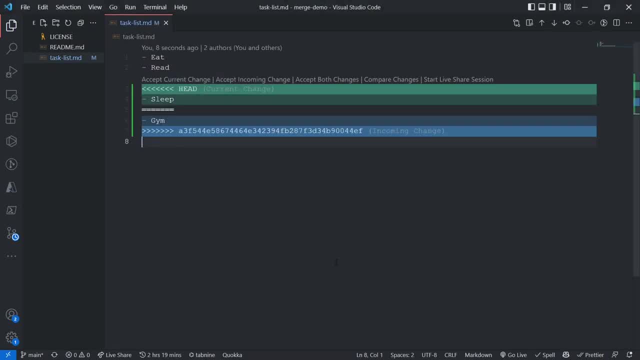 is a conflict and we are into the merge conflict situation. Now we'll be going and resolving the merge conflict situation from here. For that I'll go back to the editor again and the moment I land into the editor I see certain garbage characters over here. right, This is what most of the time 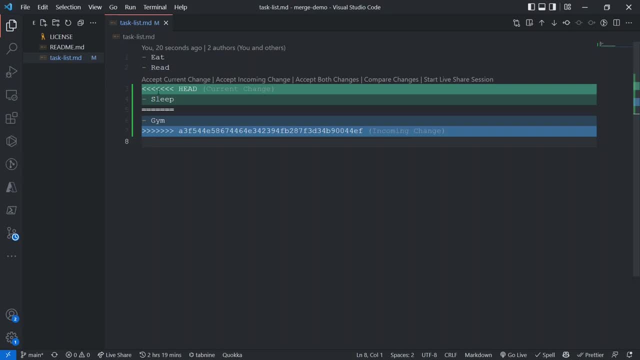 people are scared of and they think merge conflict is little bit dangerous item. Okay, so we'll tackle this. So there is a meaning of each of this character. All the outward arrow with this head keyword from here till this equals anything between. this is something. 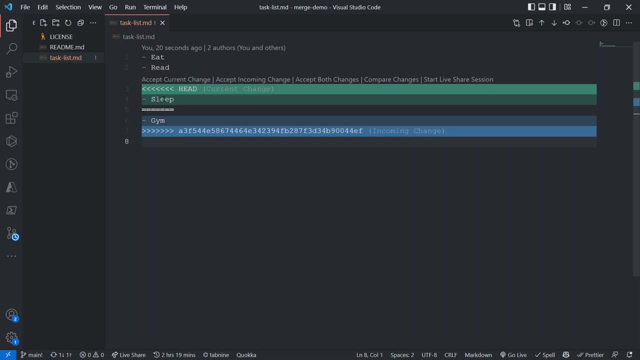 your changes, local changes that are ready to go out and go to remote. That is why this outward arrow now from this equal till this inward arrow and this particular id, this is a commit id, last commit id for this file. anything between these two is something inward. the changes are ready to come. 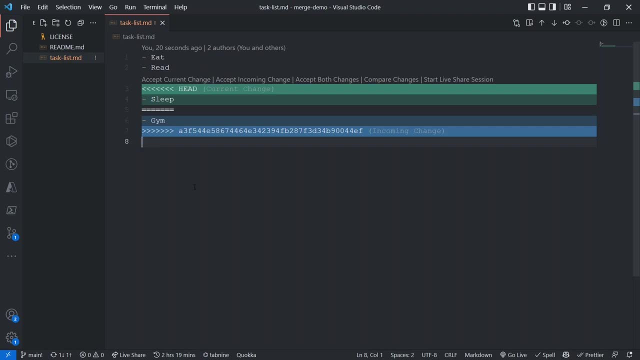 to you locally is there in the remote. okay, this is the first meaning that you have to understand. Once you understand this meaning, everything is very easy. so, from this outward arrow till this equals is your changes. from this equals to this inward arrow is changes that are there in the 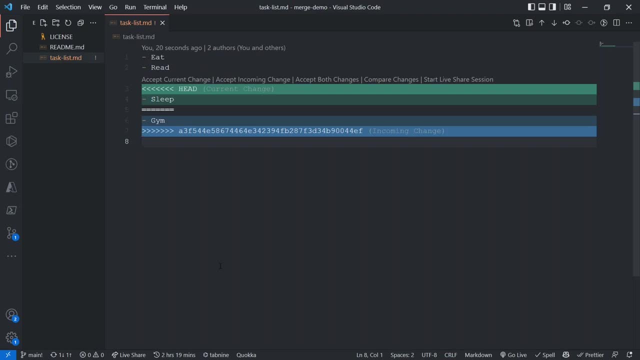 main already ready to come to you. you now you have to take a decision, based on your applications, use and usages, that what changes you want to keep. do you want to keep both of them- sleep and gym- or you want to keep just sleep or you want to keep just gym? let's say you want to keep just gym. so what you'll be doing, i'll be. 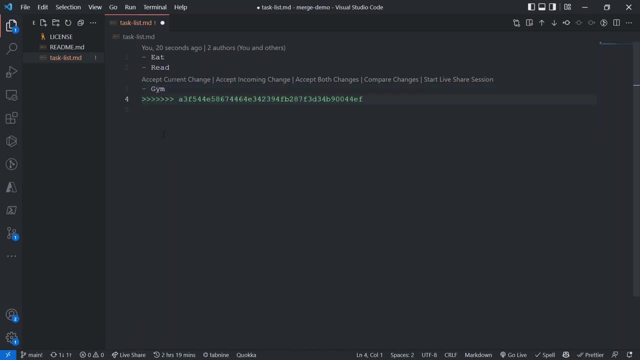 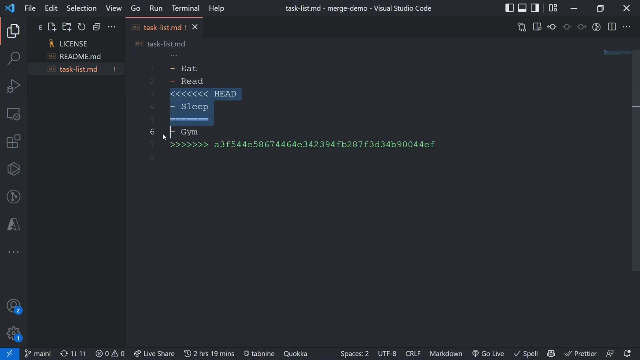 taking from here till here, i'll delete. taking from here till here, i'll delete, and then i'll be doing this. okay, this is my manual way of handling. so only gym will be there now if i want to keep, let's say, only sleep. so what i'll be doing in that case? let me revert, revert, revert, revert all the changes. 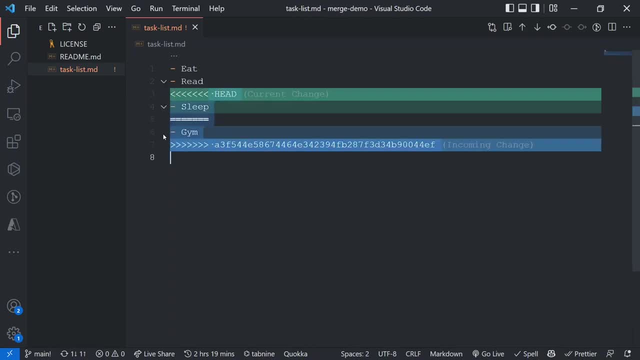 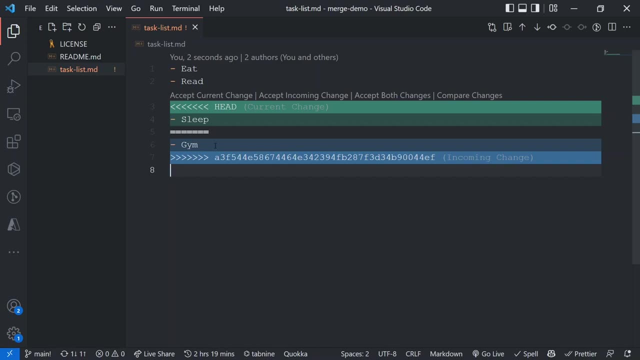 that i have done. oops, sorry, it's too much of reverting happened. yeah, so if i want to keep only the other one, so the so. appropriately, i will change it now if you are in a vs code or any other kind of git merge, merge enable editor. in that case, you can do it in the click. also like accept. 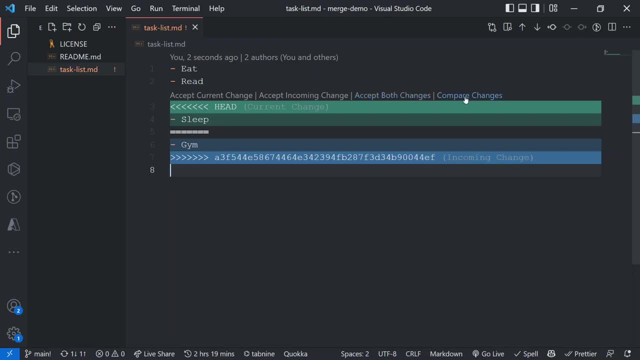 current change, accept incoming change, accept both the change or compare the change and then take. so all these handles are there with the editor, but when situation become complex, it's better to do it a bit manually, as you know, wherever required, so that you know exactly what you're doing. so let's take a case of: we want to keep both, so we. 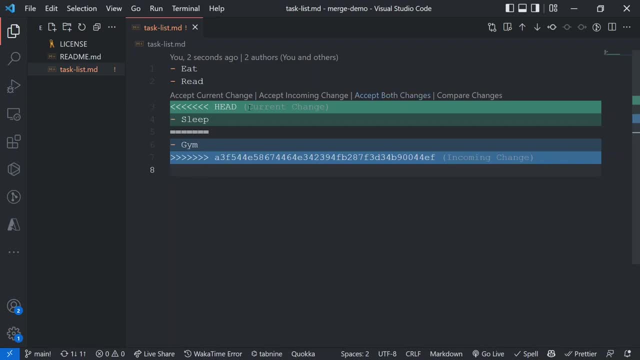 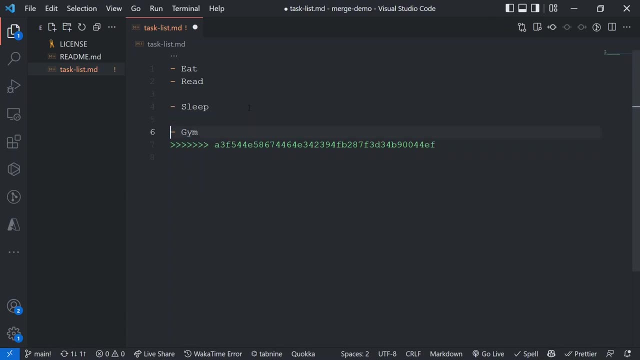 can click on this: accept both changes and accept both, or what i generally do, i go ahead and simply delete this head. this equals these things. and then i know, like what kind of formatting is required for this one. i go ahead and i save it, that's all. my changes are right. i am keeping both. so, based on what is your requirement? you? 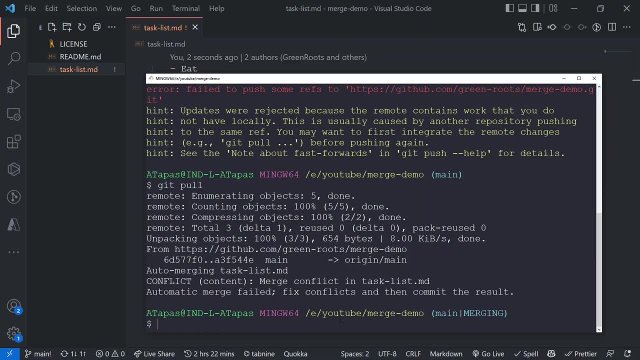 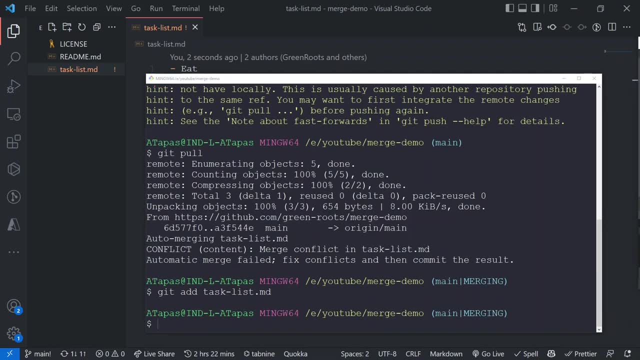 will be taking the call now. next thing is i have made a change, so what i have to do, i have to commit this change, so i'll be doing git add task clicks dot md. again, staging is done, so i'll be doing a git commit. so i won't pass any message in this case. just want to showcase that. if you don't pass, 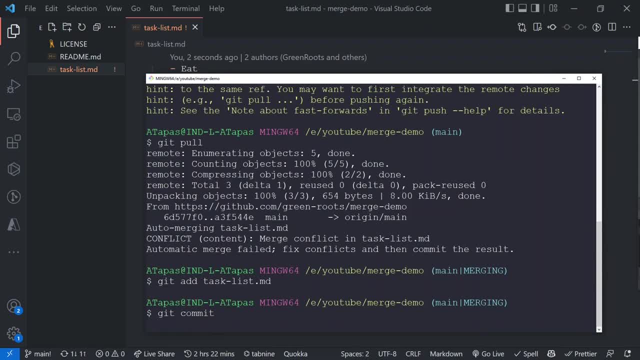 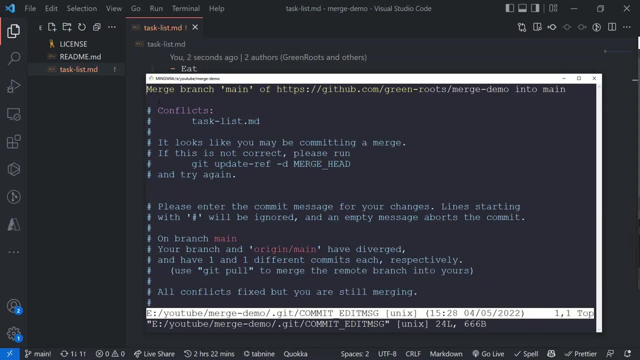 any message after doing the march conflict resolution, there will be a message automatically been added. so it will go and add that message for you. so this is the message, like merge branch from this to this. this message got added. you can also customize it by putting a message of your choice with minus n right. so that is all about so i'll. 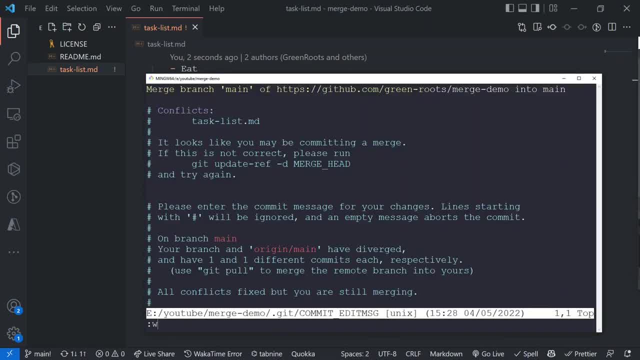 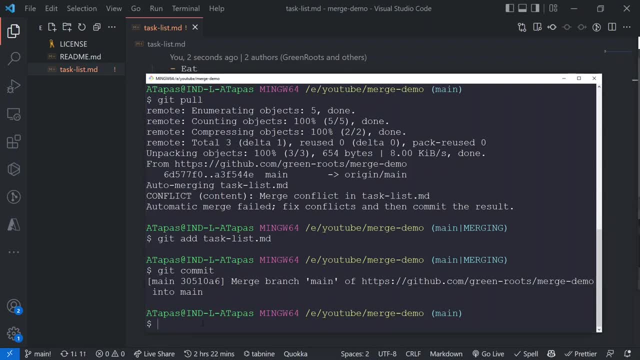 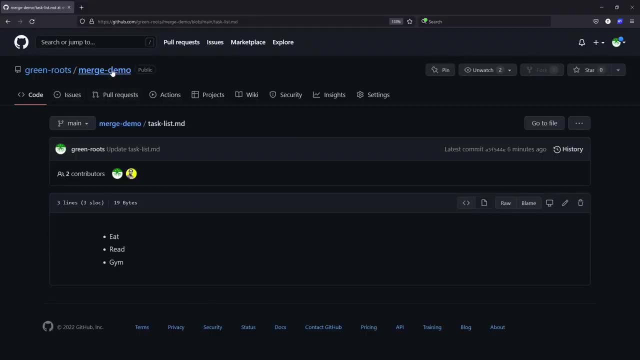 be accepting this particular one saying wq, so the commit will happen. now the final thing: what i'll be doing: i'll be pushing this change, but before i do this push, i just want to kind of go back to this view. the green roots merge info. you know aether post address and the green root. 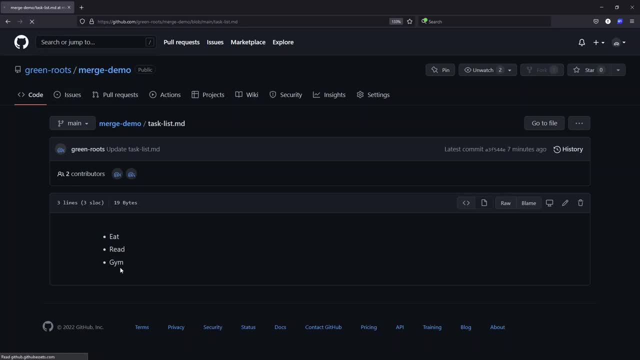 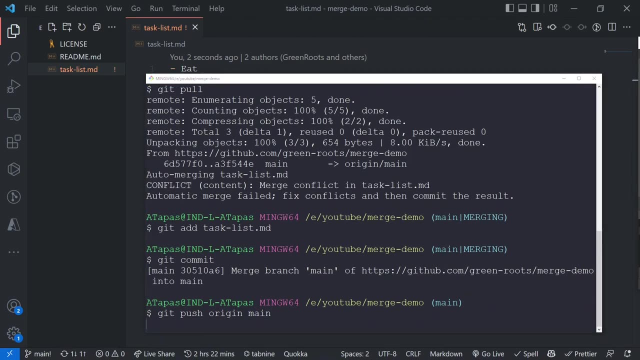 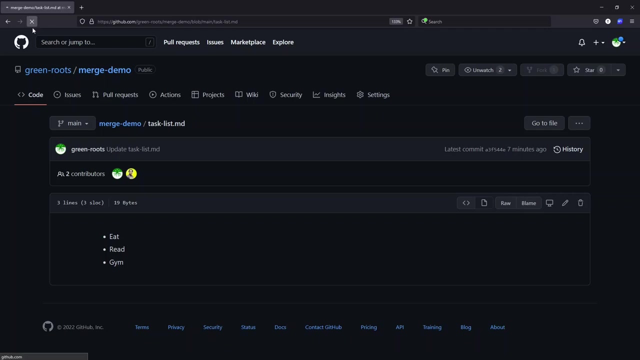 has made the change with the slip, but slip is not come yet because i have not pushed it. so i am going ahead and pushing now. my push should be successful. as you see, the push is done, so my changes are now available over here. if i just do a refresh, i see slip also. so i had decided. 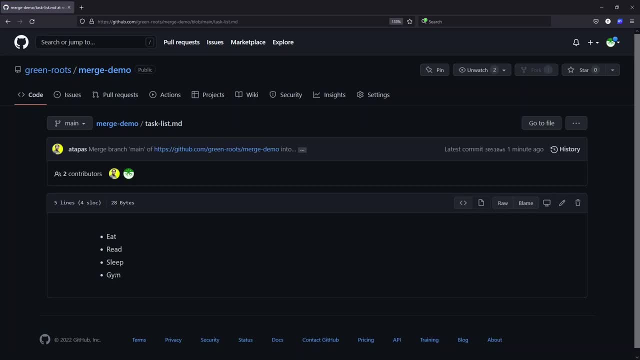 the slip should come first and then gym should come. had i decided based on my use case, gym should happen first and slip should come, i could have done the march conflict resolution accordingly. so much conflict resolution is a bit of manual effort. sometime you can use the editors. 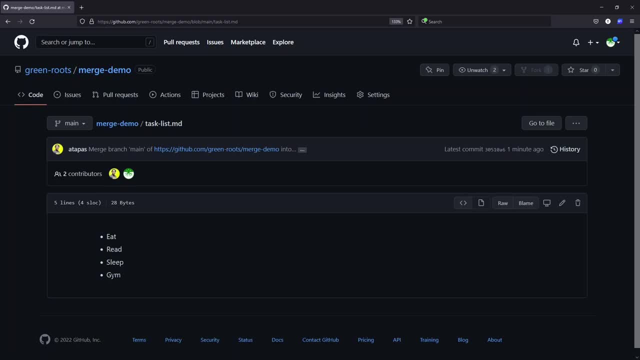 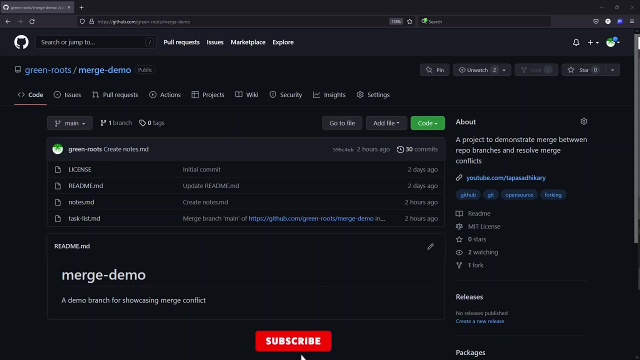 to do automation as much as possible. but the manual intervention is always good because unintentionally you don't want to delete certain things which you have taken redo later point of time. so i hope this example was useful to you. let's talk about another scenario where the much conflict resolution could be a little bit tricky. so in this scenario, what? 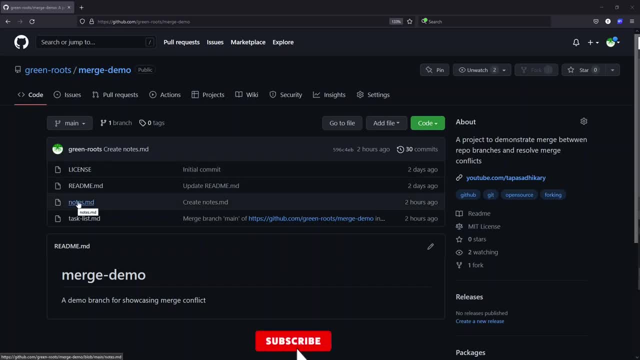 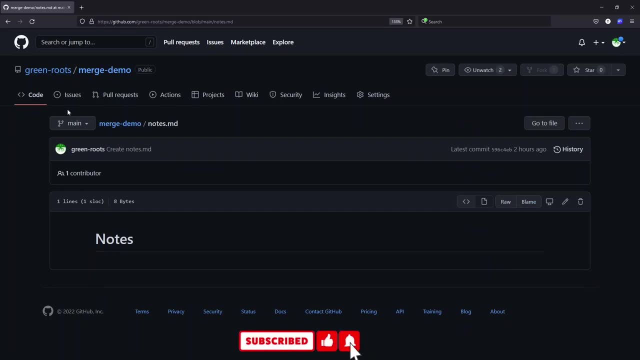 happened is like we have one file called nodesmd with probably some text in it under the same project, merge demo project. so we'll delete this file from one account, say green roots, and from another account. without knowing that we have deleted this file, we'll make some. 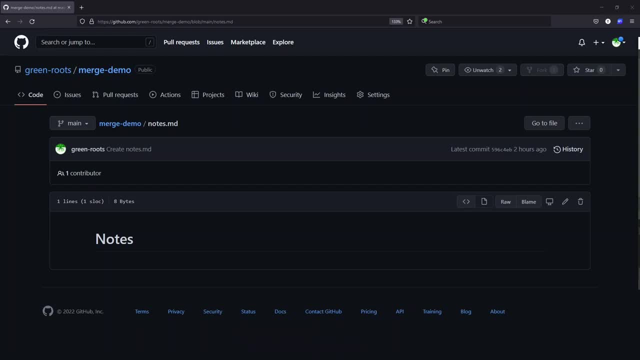 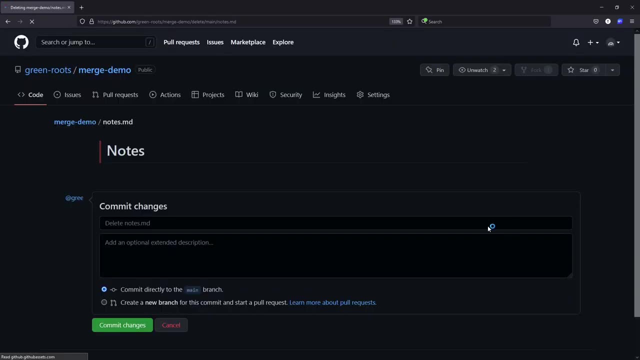 update to this particular file and see what happened. what kind of conflict that we kind of get into right. so what we do over here is like this one: i'm going to delete this file directly. so this file will be deleted and putting this comment directly. okay, so this file has been. 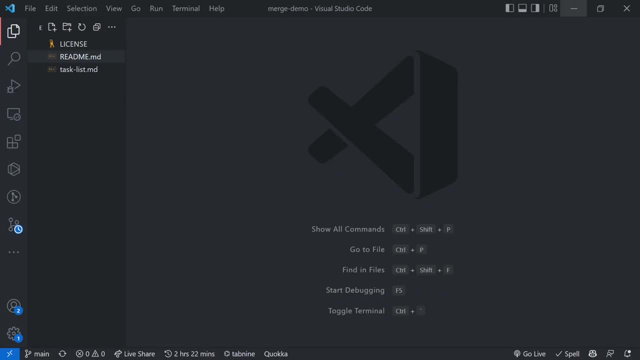 deleted. now what i'll do is, like my another account, that i have a thappas account here. this nodemd is still there, so i'll let me make some changes to it. let- okay, i am taking nodes. so fine, fair enough, i save this then. the next thing that i'm going to do over here is the regular stuff. i am going to add this: 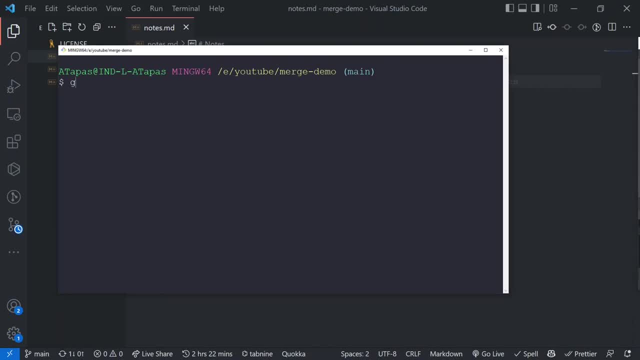 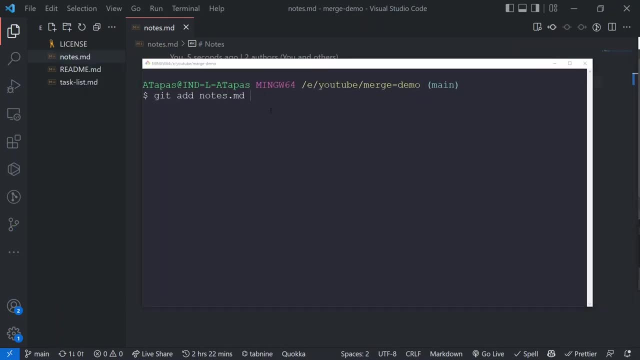 commit this and push this. okay, so let's see. so i'll do. git. add nodes dot. uh, what is the name? it's nodes, right, nodesnd. so git at nodesnd, and after that we will commit this file. let's do a commit git. commit minus m, some message: added nodes. 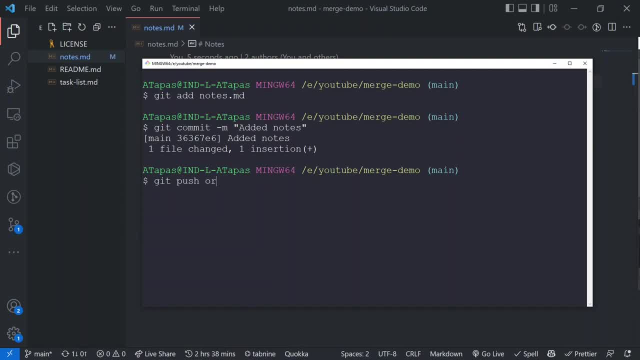 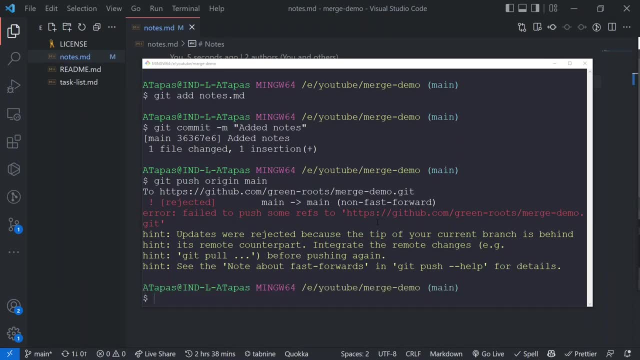 now, finally, we'll push it. so git push origin main. it says fail to push the ref because updates were rejected, because my current branch is behind, because same file has been already deleted by somebody. so there is an additional commit and my you know head, the local, whatever i am doing right now, it's behind. so the next thing, what we'll be? 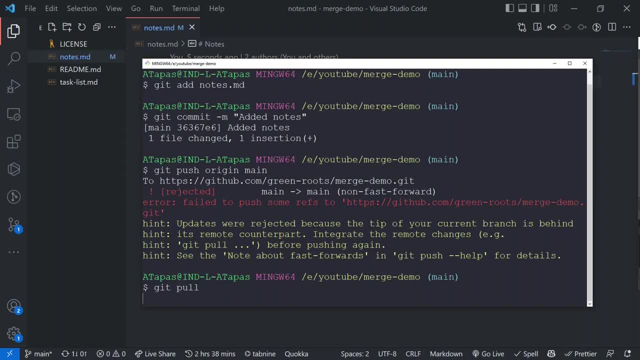 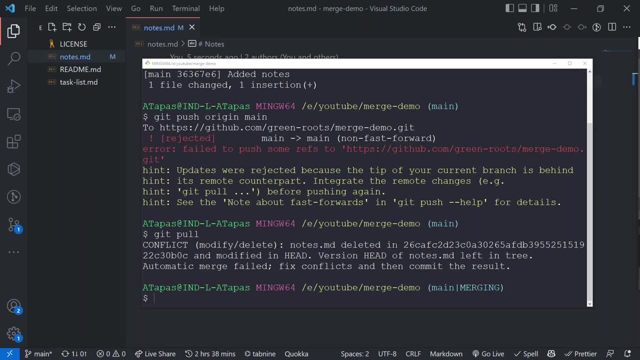 doing as a developer will be doing pool, so that i can up to date things. now see what happens. now git pull comes back with a conflict. the conflict says nodesmd is deleted, you know, and on the master or the main, and, but here you have modified, modified in head, so it's a pure. 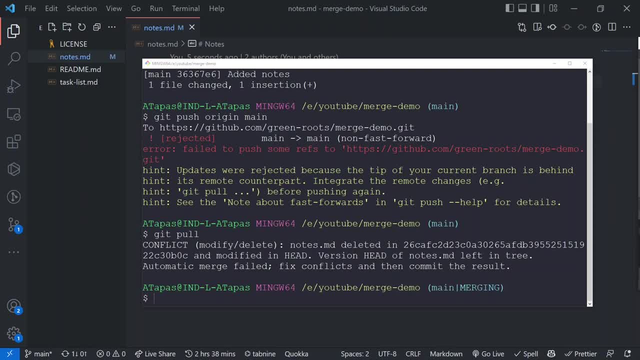 merge conflict that we have to resolve. so in this particular case, when a file got deleted, i know, by somebody, and then you are modifying the same file, you have an opportunity to decide whether you want to keep this file or you want to remove this file. is the removal done by somebody? 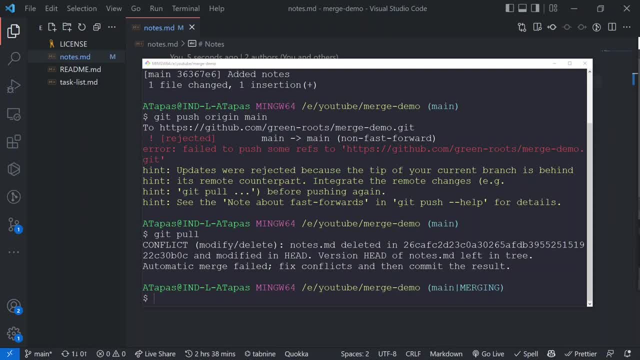 else is the right call and you just want to accept it, or it was not the right call. you know you want to kind of make sure that you want to bring back that file. so in either of the cases you have to take this call now. if you have noticed here, you know, once this merge conflict happened, it's clearly 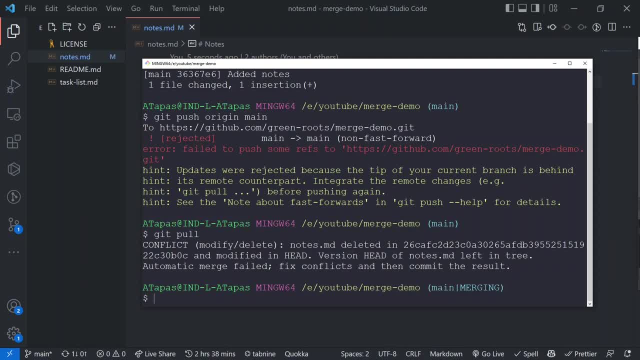 saying that it's in the merging state. right, this branch is in the merging state, it's not on, not merged it. when it is at the merge state, you won't be seeing this pipe merging at all. so, in this case, what we'll be doing, we'll be first checking the git status. let's see what is the status. come back. 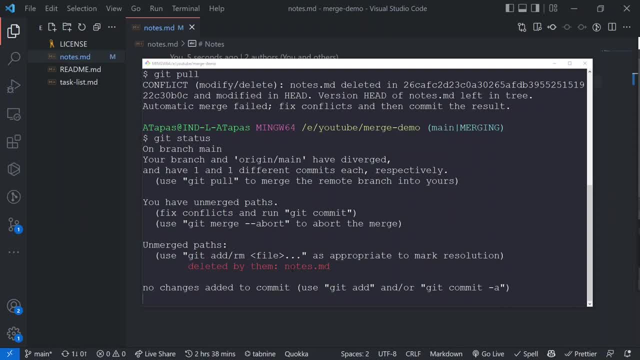 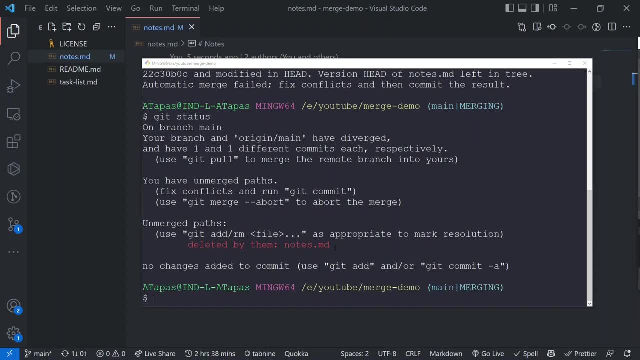 with. so you say that deleted by them means it is deleted in the report. so you can see that it is deleted by them. so you can see that it is deleted by them, but you still have it in this case. if you want to retain this file, do git at nodesmd your changes. 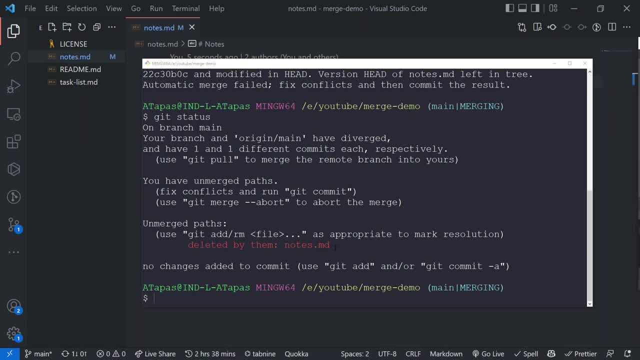 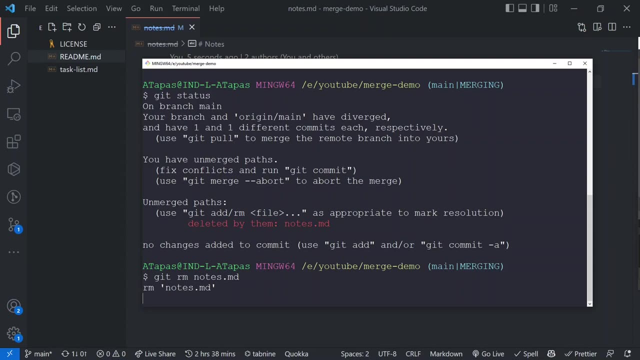 will be written and after that you can do a commit and push. but if you want to accept that it has to be removed, then do the command git rm- nodesmd- the file name. this file will be removed from your head as well and after that the regular course: you have to do a git commit and the git. 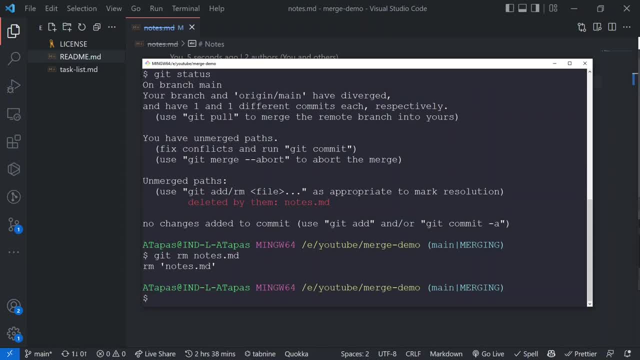 push this kind of thing scenario. you probably face in a project where you have to do a git project with the package, a logjson or yarn log file. in that cases, you know, sometimes those file will be committed to the repository but later point of time the maintainer feels that okay. 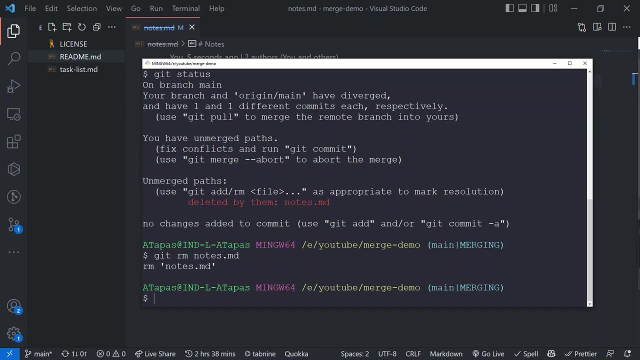 we won't be putting yarn log file into the repository and maintaining it and they delete it, but it's still there with you locally and you get some kind of conflict on the situation. so this is the time where you have to really, really make sure that you do the right things. okay, so let's do a. 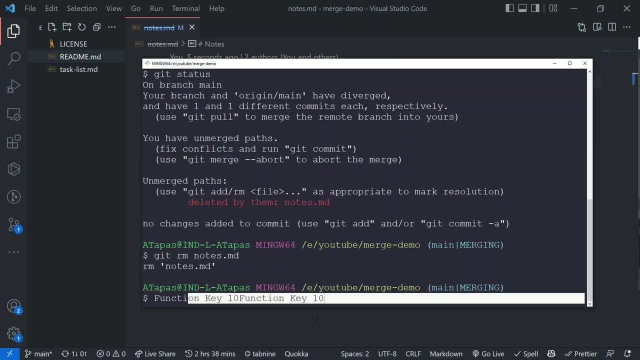 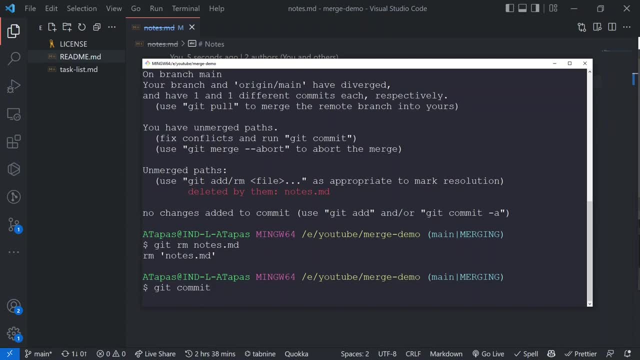 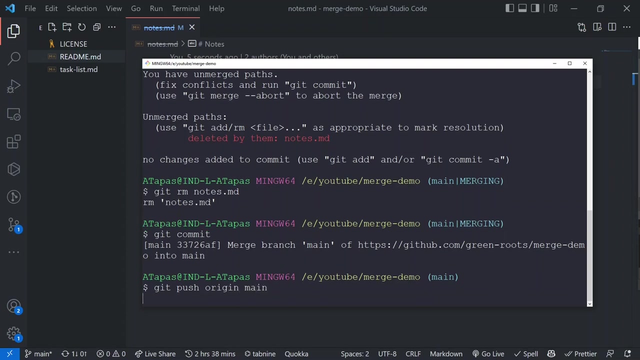 commit and push. first we'll do a commit. okay, let's remove this git commit. we'll get the default merge message over here. that's what we get. so we accept that message. with wq, now we will push, and now this push will be successful. here you go, the 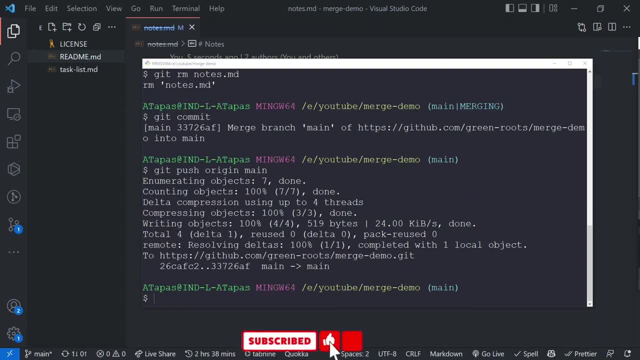 push is successful. so we have spoken to very vital scenarios in terms of merge, conflict and how to handle them. if you faced any other scenarios other than this, please comment in this video and i would like to kind of think through, understand and if you need any help on those.